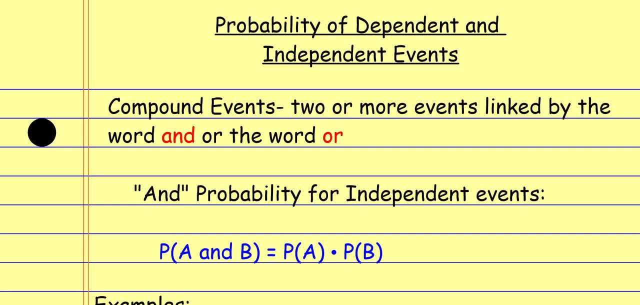 talk about compound probabilities. Compound probabilities are basically when we have more than one thing that we're looking at at the same time and we either want both of those things to happen, so we link it with the word and, or we want one or the other of those two things to happen. 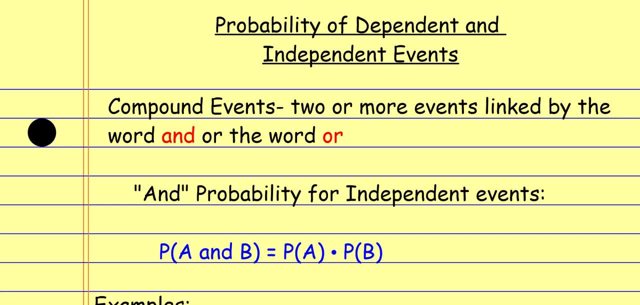 so we link it with the word or. okay, So compound events, two or more events linked by the word and or the word, or For dependent and independent events. we're going to focus on those and probabilities. all right, So these are all compound probabilities because we have more. 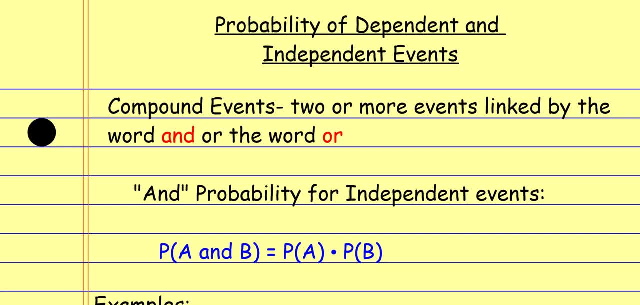 than one thing that we want to happen, all right. And we either want both things to happen, so we say and, or we want one or the other, so we say or. So with the and probabilities. so this is for independent events. we just say: if I want the probability of A and B, 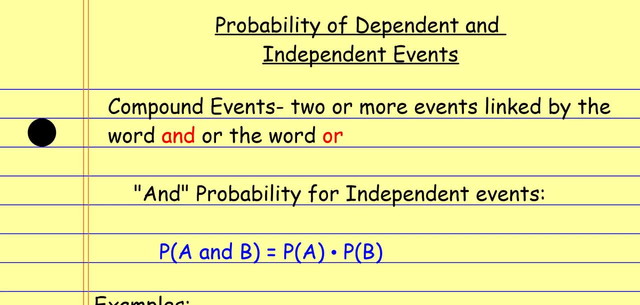 I take the probability of A times the probability of B, all right, And again, this is just two things. so if I say, hey, what's the probability of the first thing happening Now separately, what's the probability of the second thing happening? Well, if I want the probability of both of those things, 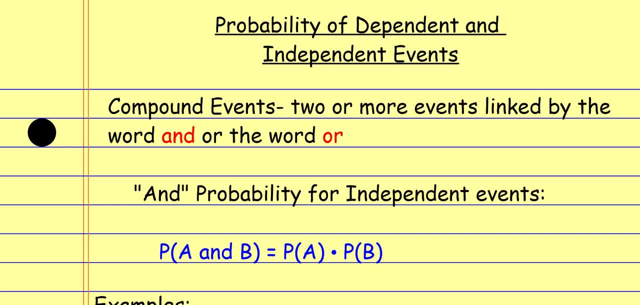 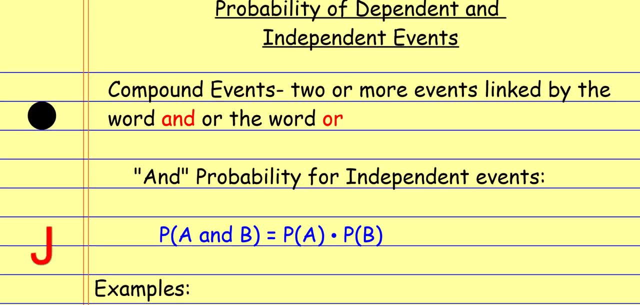 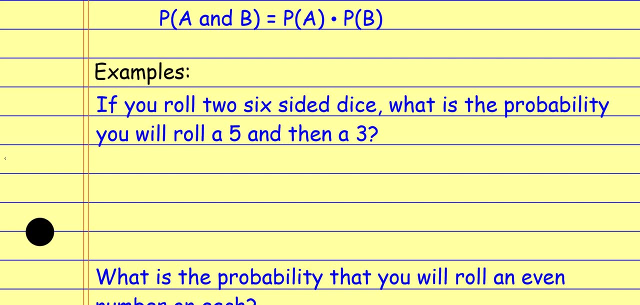 happening. I want the probability of this thing and this thing. I just take the two separate probabilities and I multiply those two fractions together. okay, For example, let's look at something like this guy: If you roll a six sided dice- or really it should be a six-sided die- what is the probability that you will roll a five? 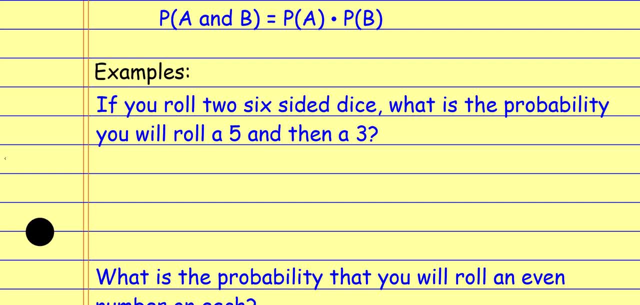 and then roll a three, And so again, I just have two separate probabilities happening and we're linking those two things with the word, and so I just say, hey, what's the probability of rolling a five? Well, that's one out of the six options, so the probability of rolling a five is one out of six. 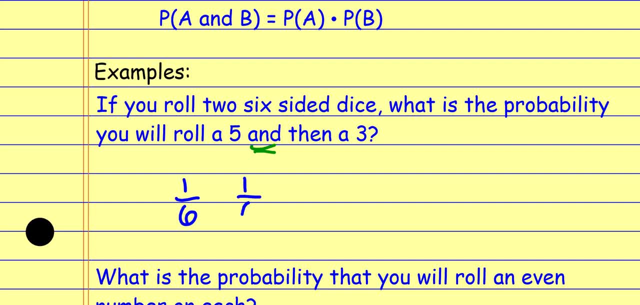 And then we say, okay, what's the probability of rolling a three? Well, there's one of those out of the six options, so that's also one out of six. So if I wanted the probability of rolling a five and rolling a six- sorry, rolling a five and rolling a three- I multiply these two probabilities. 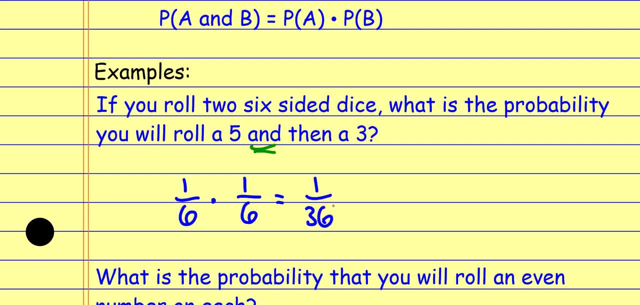 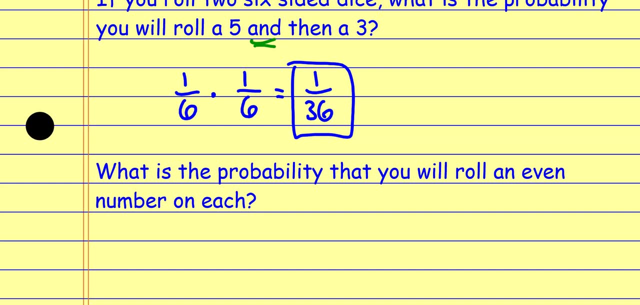 so that gives me one over 36.. Remember, when you multiply fractions, it's numerator times the numerator, denominator times the denominator, and that's it. If I look at the next one, it says what is the probability that you will roll an even number on each. So I'm rolling two different. 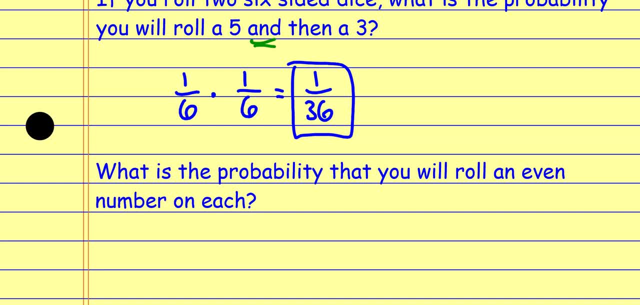 so I'm rolling a pair of dice here. I want to know the probability of rolling an even number on each. As you look through here, the word and is not listed, but the word and is implied here. If I want to roll an even number on each, that means I need an even number on the first die and an even. 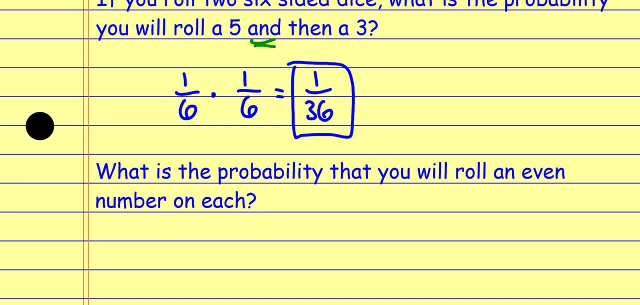 number on the second die, and so that word and is implied. It's not necessarily about the word, it's about the situation. Do I want both things happening? Yes, it's an and all right If I want one or the other. it would be an or So for this one to roll an, even on the first die. so again, 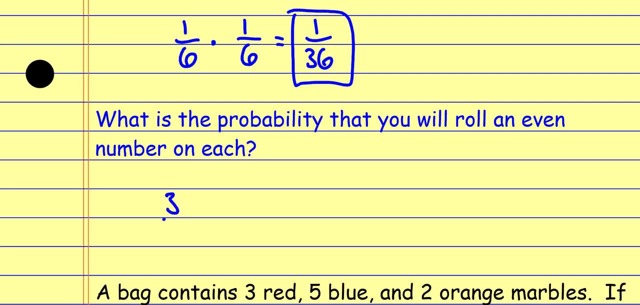 an even number, there are three even numbers when you roll that thing, so it's three out of six. And then the probability of rolling an even number on the second die is also three out of six. If I want both of these things to happen, if it's an and probability, I multiply the two. 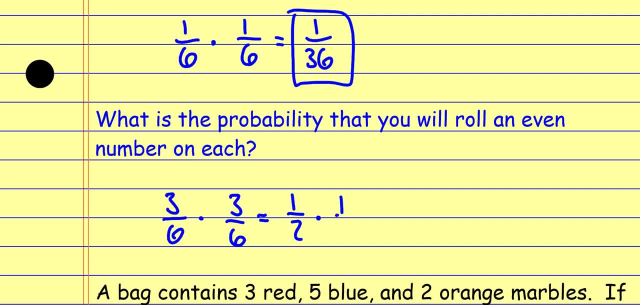 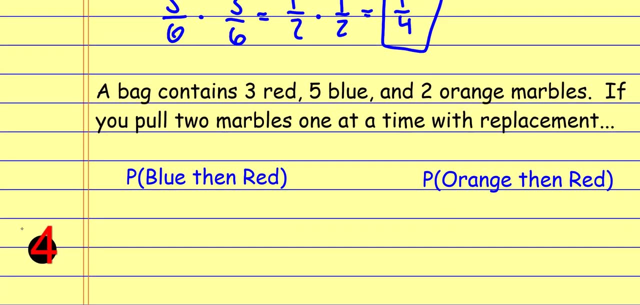 and I'm going to reduce each of these fractions. first, That's one half times one half, so the probability becomes one fourth. So I'm just working out the probability of each, but the and tells me to multiply those probabilities. But look at this one. it says a bag contains three red, five blue and two orange marbles. 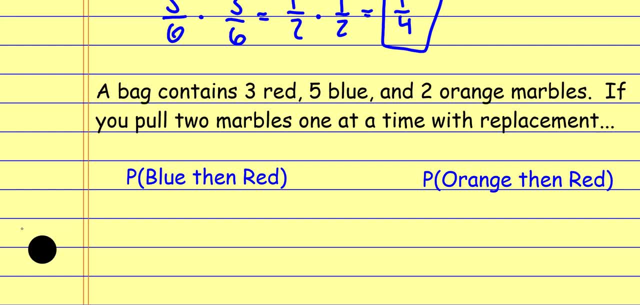 If you pull two marbles, one at a time, with replacement, what's the probability of blue than red? And then it also asks us, what's the probability of orange than red? And the key to this thing right here is: with replacement. what does that mean? Let's talk about that. 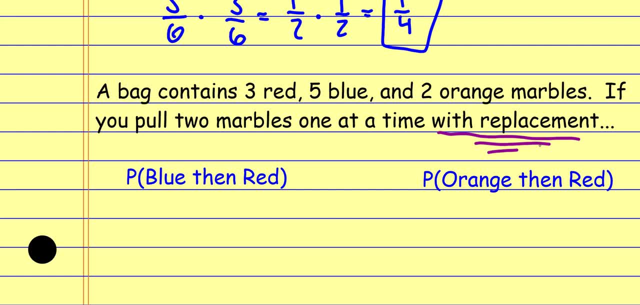 With replacement means. I reach in there, I pull out a marble, I see what it looks like, but then I put the marble back. I replace the marble. I pull out the marble, I replace the marble, I put it back in the bag and that makes these independent events See, independent events are. 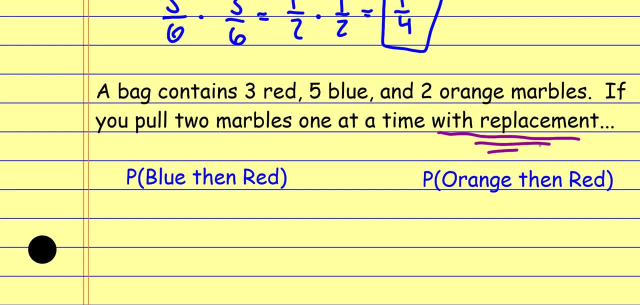 events that do not affect one another. Like in the previous examples, we were always allowing two separate die. Well, those don't affect one another, because what I get on one doesn't affect what I can get on the other. And here, if I didn't replace that marble, it would change how many. 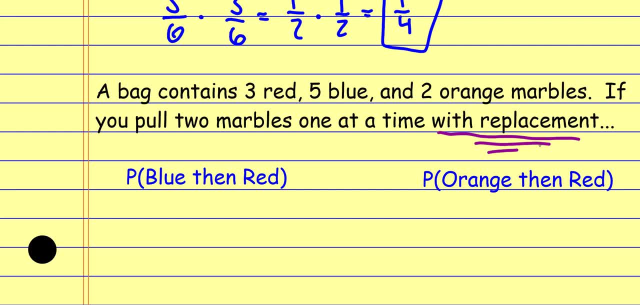 marbles are in the bag. so that means the first thing would have an effect on the second thing, So that with replacement is important. I pull the marble out, I look at it, I put it back in. So when I look at this first example, 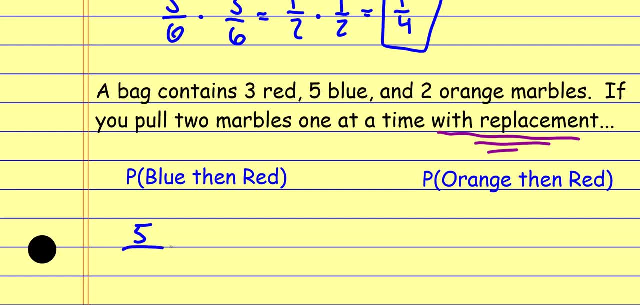 the probability of blue. there are five blue marbles out of a total of ten marbles And then the red marble. so I pull the blue marble out, I put it back in. There are three red marbles out of a total of ten marbles and it's still ten because I put 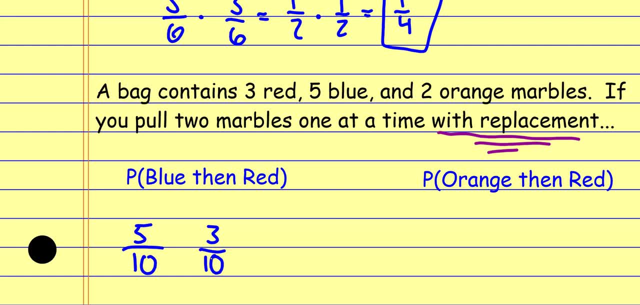 that first marble back And again the word and is not written here, but it's implied. I want a blue marble and then a red marble. okay, We would never say a blue marble or then a red. that doesn't make sense, all right, But think about the situation. I want both of these things. 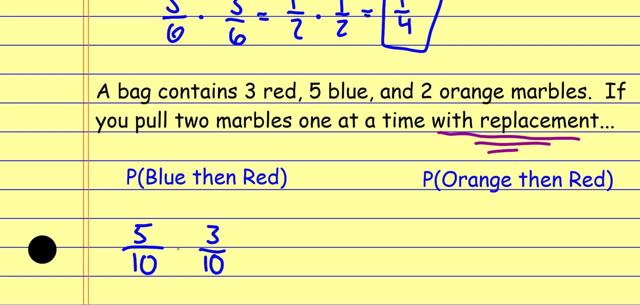 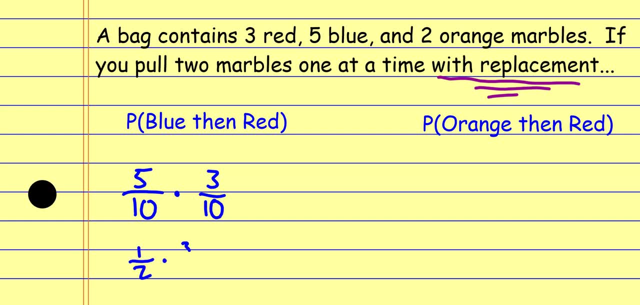 to happen. I want a blue marble and a red marble, so that's an and probability. I'm going to multiply And once again I want to simplify this fraction first. So let's see that's a one half times a three over ten. so that gives me a three out of twenty. So the probability of getting those two. 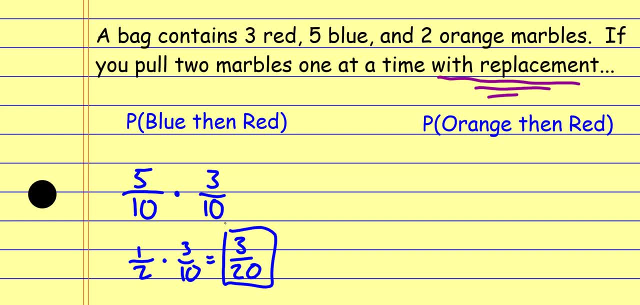 things is a three out of twenty, all right. The next one, an orange marble, would be a two out of ten. The probability of a red marble would be three out of ten. And again, the reason it's three out of ten is because I put that first. 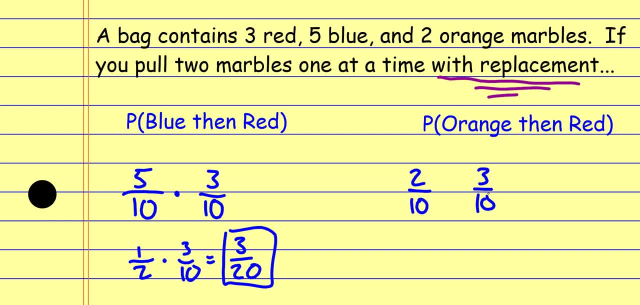 marble back after I looked at it. so there's still ten marbles in the bag That's going to become important later. The word and is implied here. I want both of these things, so now let's reduce and do our multiplication. So that gives me a three out of fifty. 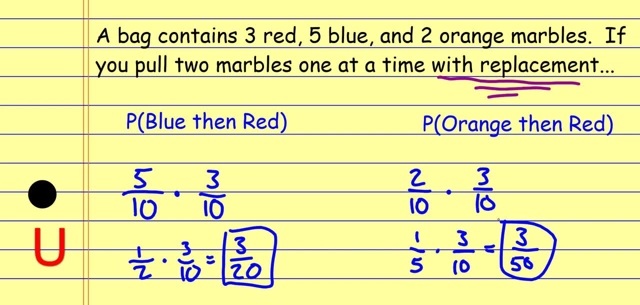 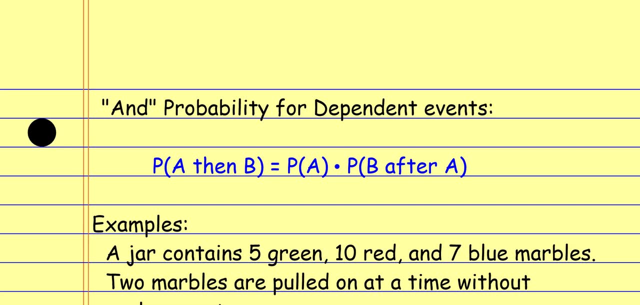 But again not much different than what we were doing. I'm still working out each probability individually, but now, because the and I want both of those things to happen, I multiply the two. Let's talk about dependent events. The difference between dependent and independent is really just. 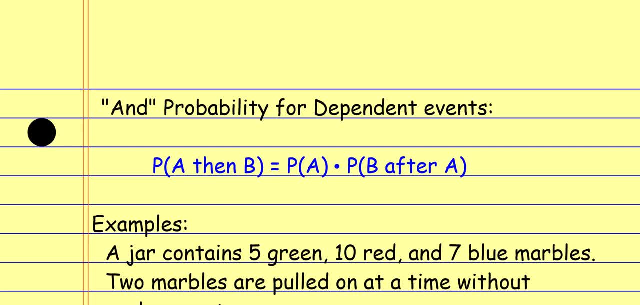 a matter of a little bit of imagination. We have to imagine that the first thing happened and that's it. It's literally still the same thing, but we have to think about the situation, We have to imagine what's going on. So, and probability for dependent events is the 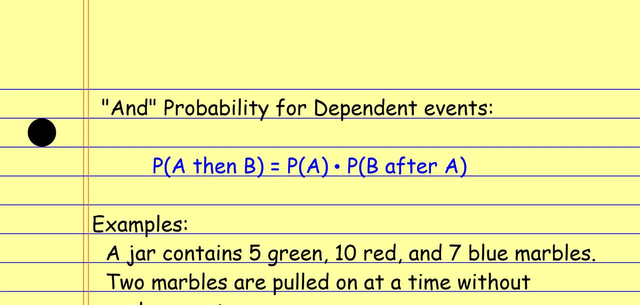 probability of a then b. We have to do the probability of a times the probability of b after a, And that's the same thing we were just doing, except with a little bit of imagination. So what it's saying is: we take the probability of the first thing, No problem, That's not any. 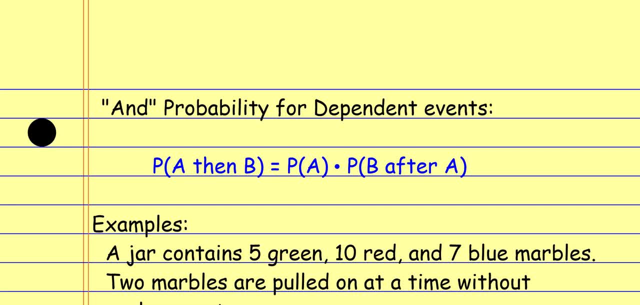 different. But then I imagine that that first thing happened. and if that first thing had already happened now, what's the probability Of the second thing happening? because they're dependent events. whatever happened first affects what's going to happen second. It changes the possibilities in terms of the outcomes. 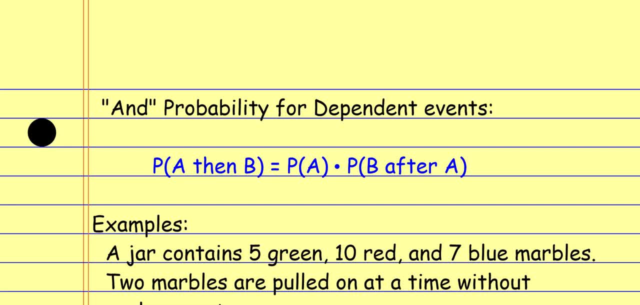 See the previous example. independent, they have no effect on one another. so I need to imagine what happened. But here, if they're dependent event, it means that the first event happening has a direct effect, a direct impact on what could happen for the second event. So I have to imagine. 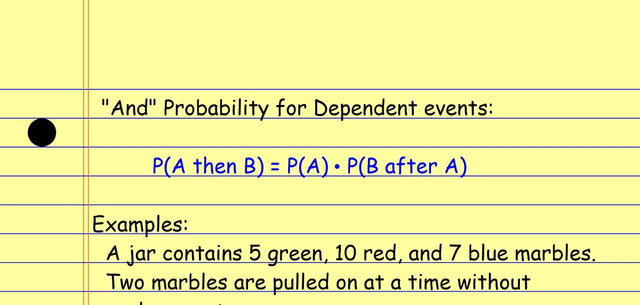 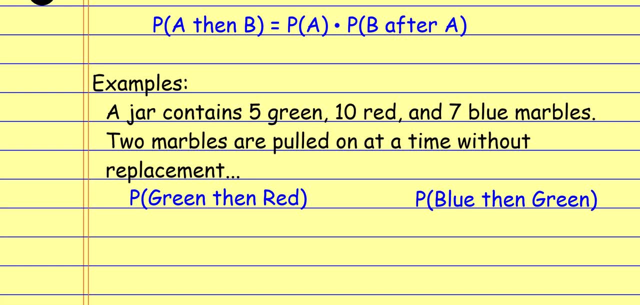 that first thing has happened. For example- let's take a look at an example here. It says: a jar contains five green, 10 red and seven blue marbles. Two marbles are pulled, one at a time. Started a little typo there: One at a time, without replacement this time, And so that's. 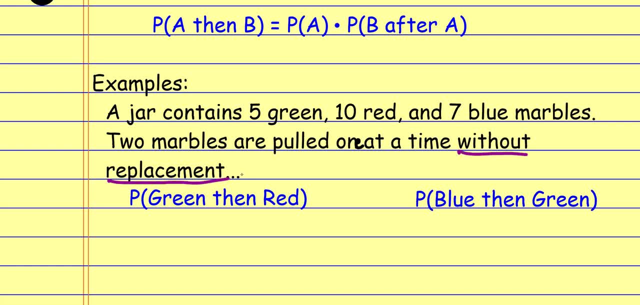 the key here, Without replacement, means once I pull that first marble out, I do not put it back in the jar. So here the probability of green, same thing that we've always done. There are five green marbles out of a total of 22 marbles. So the 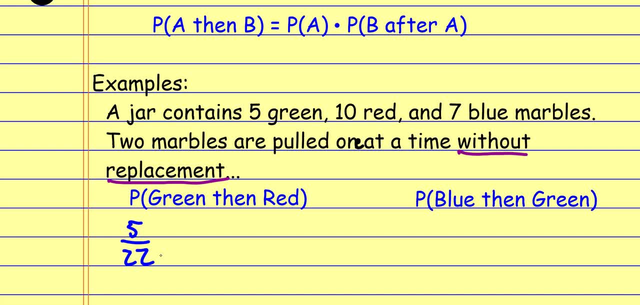 probability of green is 5 out of 22,. but now I have to imagine that that has happened. I have to imagine that I pulled a green marble out of that jar. And if I pulled a green marble out of that jar, if I use my imagination here, that means now there's only 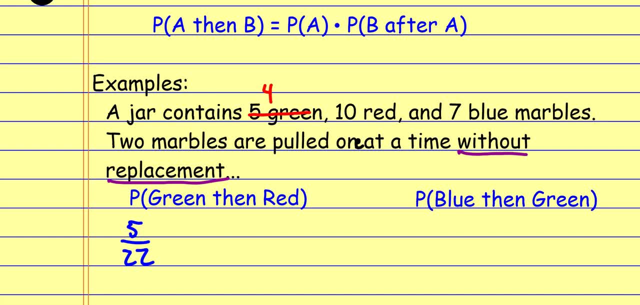 Speaker: 2: 0.50 green marbles left right. So when I do the probability of red, there are still 10 red marbles, but because there's only four greens left, I only have 21 marbles total left in the. 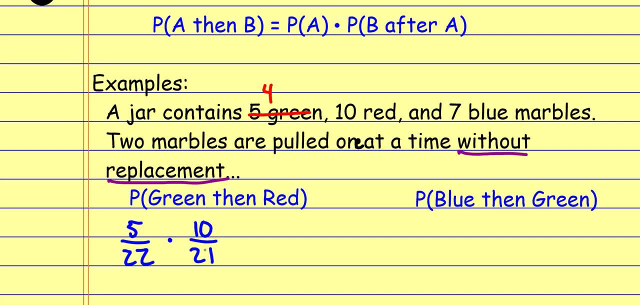 jar And see, that's the difference between dependent and independent. okay, The dependent: here the values changed because of what happened. okay, As opposed to independent, where they don't affect one another. And of course, I can cross, reduce, Remember whenever we have fractions. 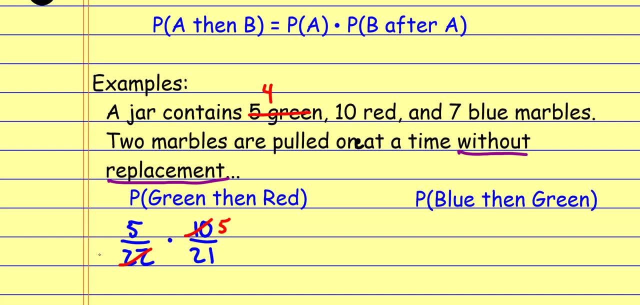 reduce these guys. they're each divisible by two, so that's a 5 over 11.. And I think that's all that simplifies. So now I multiply straight across. that's a 25 over. it looks like a 231.. 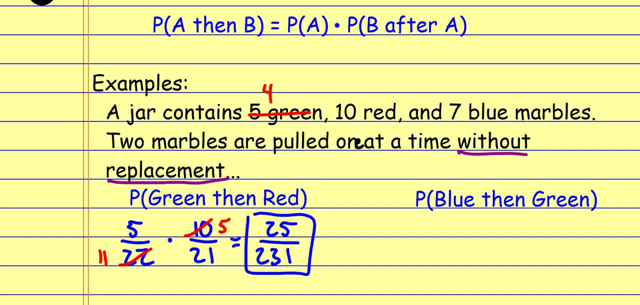 So 25 over 231, okay, But now I got to hit the reset button on this one. all right, So this one, the probability of a blue marble, then a green marble. So the probability of a blue marble. let's see there are seven blue marbles. 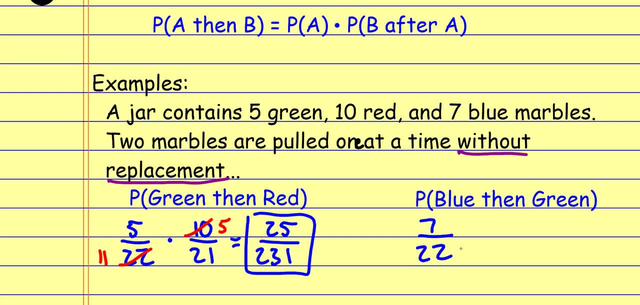 Out of once again 22 total. But now I have to imagine that this first thing has happened. So imagine I took a blue marble out. now there's only six of them, right? So now the probability of a green marble: well, there's five green marbles, but now there's only 21 marbles total. 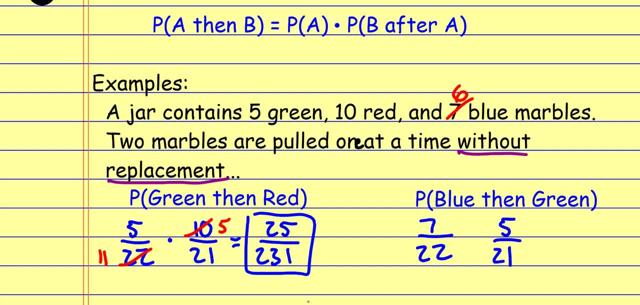 I don't know why I put an equal sign there. This is an and probability, so I want to multiply. And now, of course, I can reduce the seven and the 21,. one reduced to a one and a three. and now I multiply. 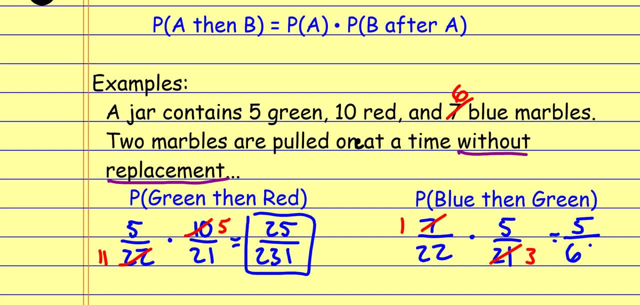 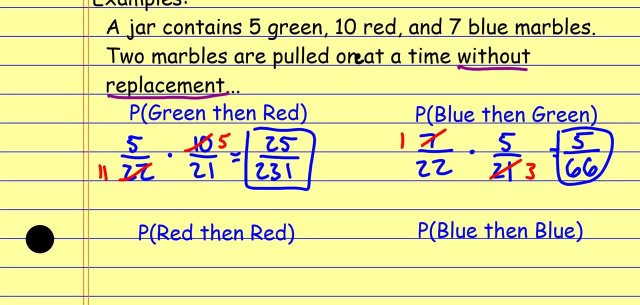 So now I multiply straight across, that gives me a five over 66.. Okay, But again, it's just a little bit of imagination. Let me erase that. hit the reset button. again This one, the probability of red, then red. So again the probability of a red. 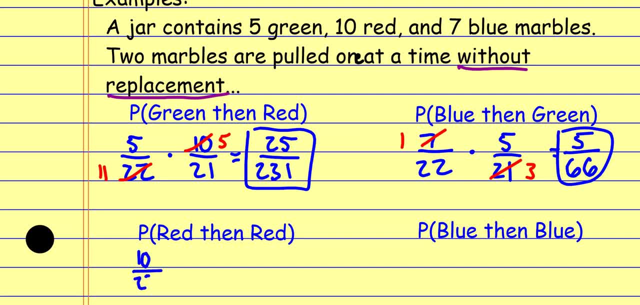 marble. there are 10 red marbles out of 22 marbles total. But now imagine that I took out one of those red marbles. That means there's only nine left. I took one out And now the probability of a red marble is nine because there's nine red marbles out of 21.. 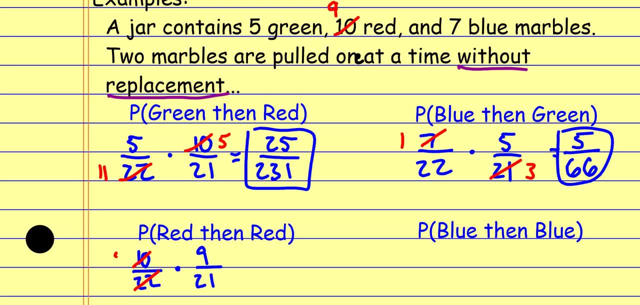 And once again I can reduce. The 10 over 22 reduces to a five over 11.. The nine over 21 reduces to a three over seven, And now I multiply straight across, that's a 15 over 77.. But again, I'm just multiplying fractions. Okay, Again, let me hit the reset button here. 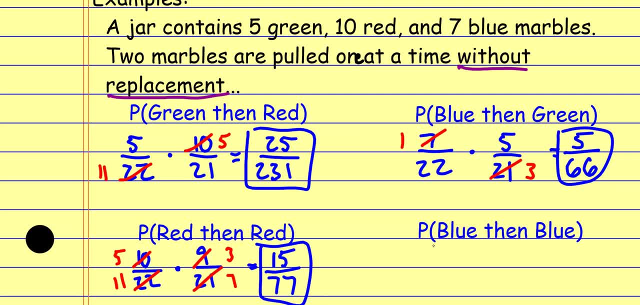 All right back to the start. So now I have a blue marble. that's seven out of the 22.. But now imagine that I've taken out one of those blue marbles. So now there's only six blue marbles left. So now the probability of a blue. 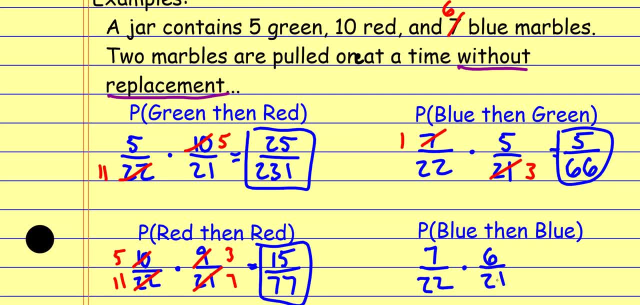 marble is six out of 21.. I have to use my imagination. I have to pretend that that first thing happened. And now I can start reducing. I can cross-reduce: that's a one and a three, The six and the 22,. I can reduce to an 11 and a 32.. And now I can start reducing. I can cross-reduce. 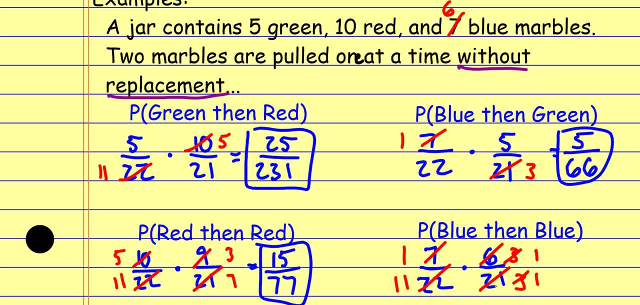 that's a three. Oh, and then I could cross out these threes to a one and a one and then multiply straight across. You can, when you're multiplying fractions, you can multiply straight across and then reduce the fraction, But that ends up being more work. 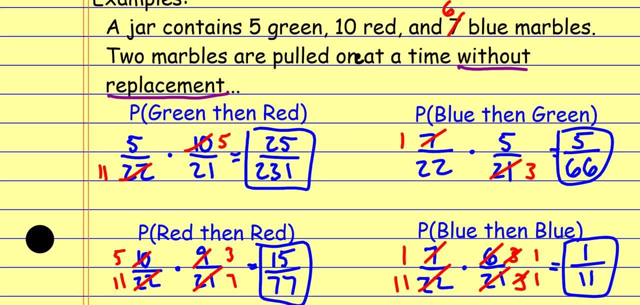 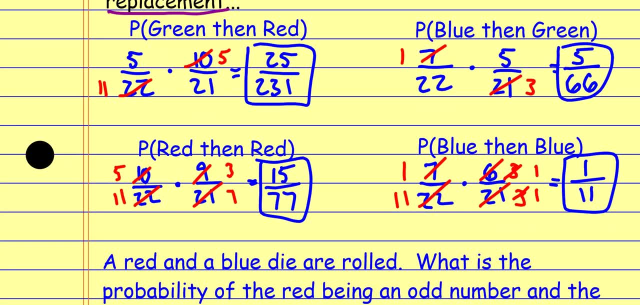 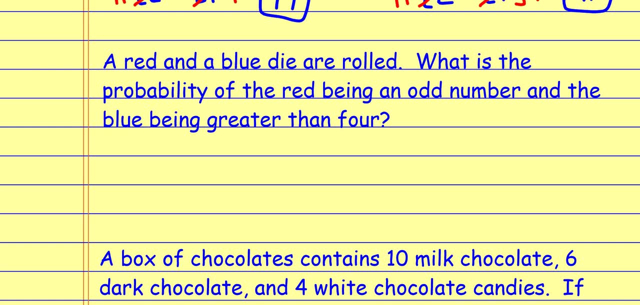 because you have larger numbers to reduce. You can always reduce individual fractions. You can always cross-reduce when you're multiplying fractions, but only when you're multiplying fractions. This one: a red and a blue die are rolled. What is the probability of the red being? 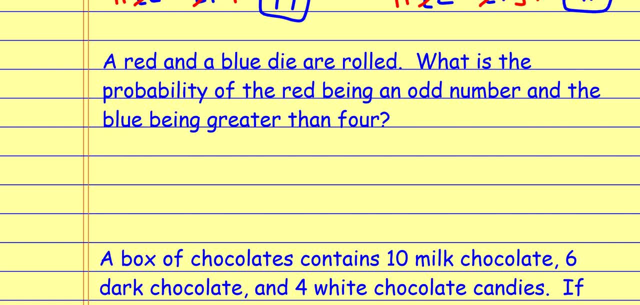 an odd number and the blue being greater than four. So once again, I want both of these things to happen. It's an and probability And these are independent events. What I get on the red die does not affect the possibilities for what I can get on the blue die. So the probability for the red die. 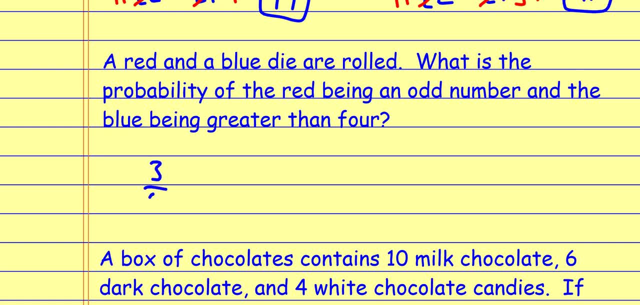 let's see odd number, So that's three out of six, And then the blue die. I want a number that's greater than four. There are two numbers that are greater than four, five and six out of the six possibilities, And then I want to multiply these And once again you can reduce these fractions. 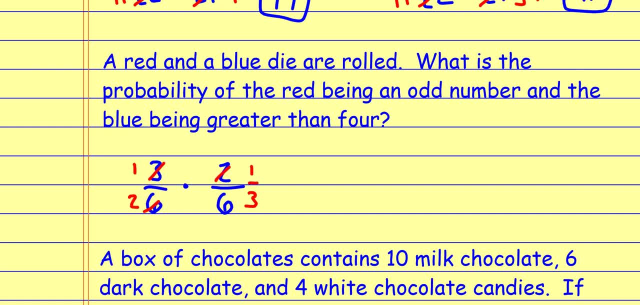 That's a one half, This guy is a one third. And now multiply straight across, The probability is one out of six. I come up with the probabilities and then the and tells me to multiply. All right, And again, if you just use your imagination, it kind of takes care of whether this thing is.